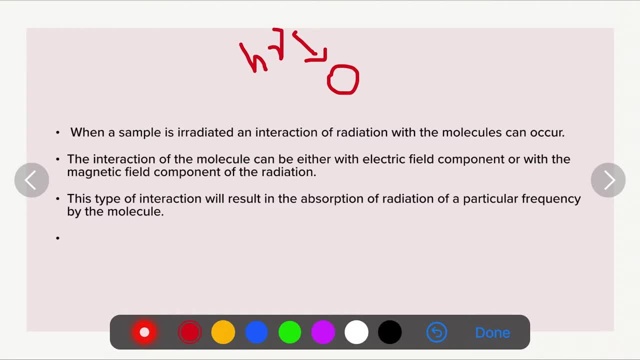 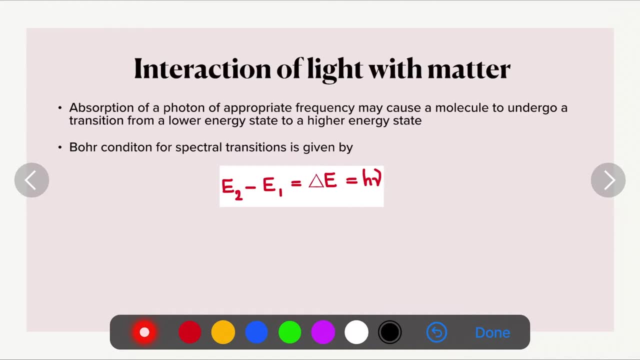 In such interactions the molecule absorbs a particular frequency of radiation. For example, if a photon absorbs a frequency called nu, it will draw the energy variable hnu. So if the molecule absorbs such an amount of energy, it will be able to produce a certain 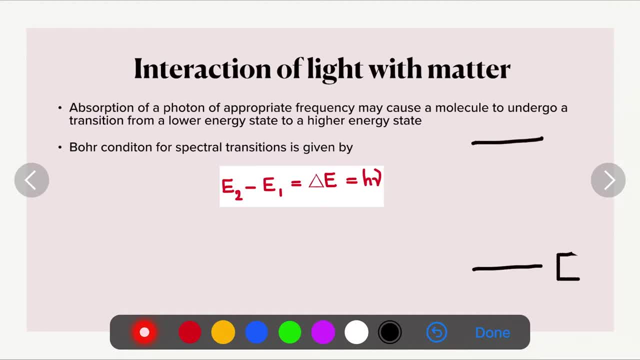 reaction transition from a lower state to its higher energy state. If we consider the lower energy state as E1,, it will undergo a transition from E1 to the higher energy state, E2.. So if there is a transition from E1 to E2, there is a condition. 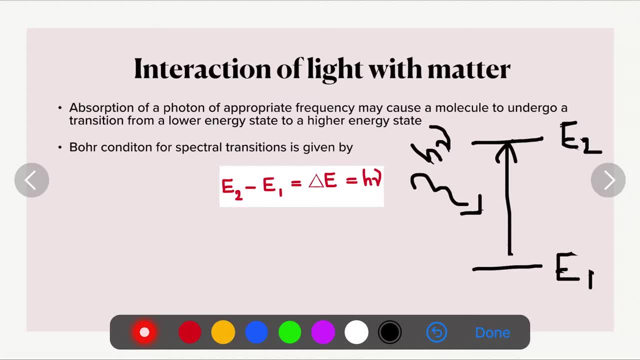 Before the тойne the flow current is equal to the contact current in the column of the molecule. This is theannot must to be absorbed sourcesso this is known as the Bohr condition for spectral transition, that is, E2 minus E1. 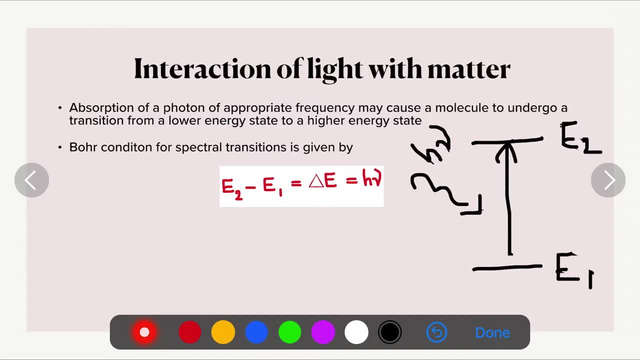 which is equal to h, equals to hал. So in name to our molecule, the flow current is nutson allowed to thenier the demon r modal which we call as non matrilocal, denn observed in the' I'm going to violent is crochet for. 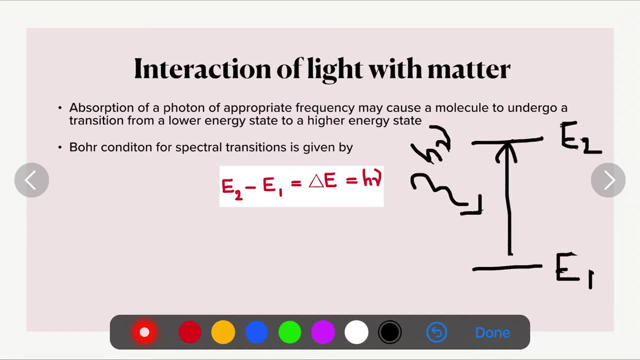 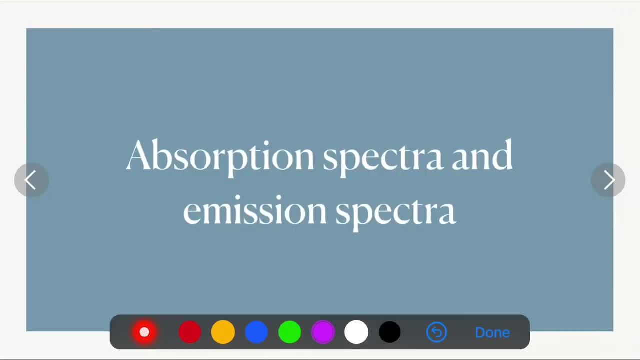 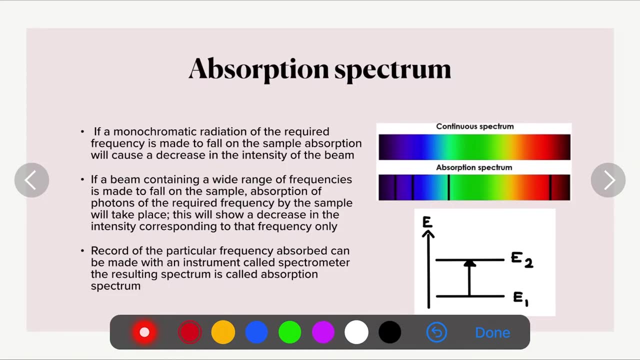 only then the transition from even to e to v will take place. Now let's discuss absorption spectra and emission spectra. Here you can see a continuous spectra as well as absorption spectra If we irradiate a molecule with a wide range of frequency light. 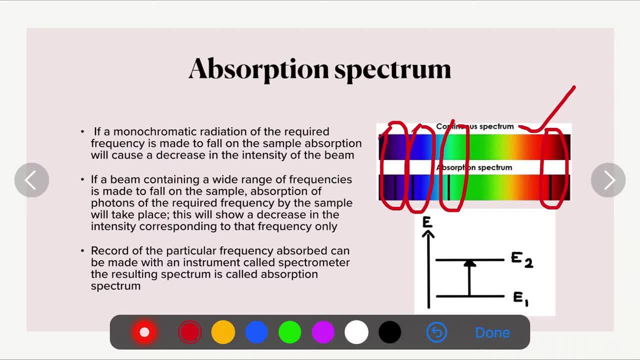 it will absorb all the energy required by that molecule, So that area will be shown as a dark line. This is because the molecule absorbs the light from that frequency. Now, instead of a wide range of frequency light, if we are following a single frequency, ie monochromatic radiation on the sample, 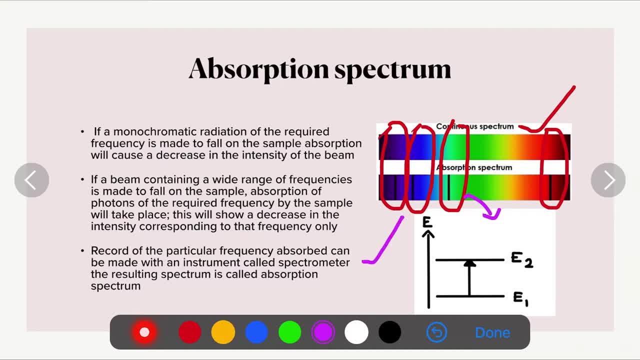 the light that is transmitted to us, there will be a slight decrease in the intensity of that light. That means when the radiation comes into the molecule, a certain amount of energy has been absorbed, So the rest of the energy is transmitted to us. 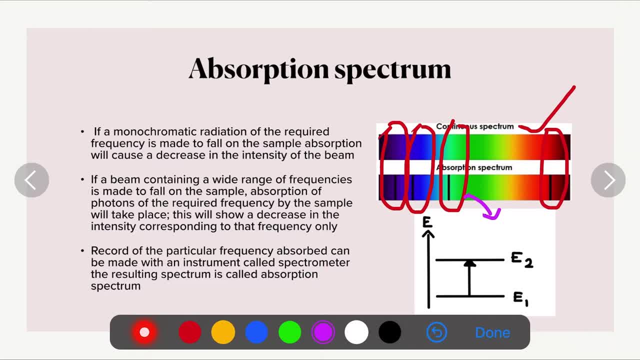 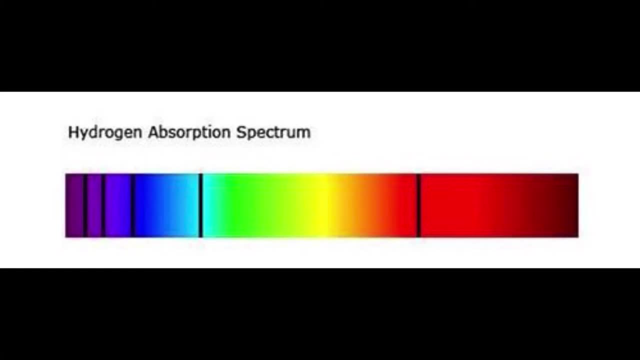 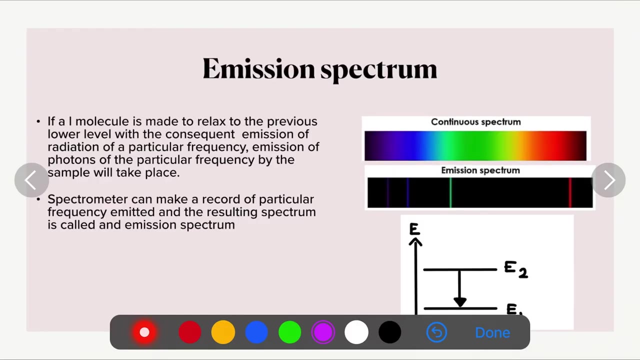 So, after taking two cases, we can record the wavelength or frequency absorbed by the molecule With the help of an instrument called spectrometer. this is called the absorption spectra. For this, a molecule at a higher energy level has to emit a certain amount of energy to reach its lower energy level. 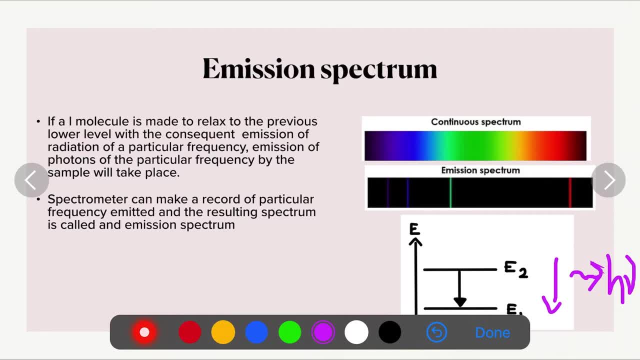 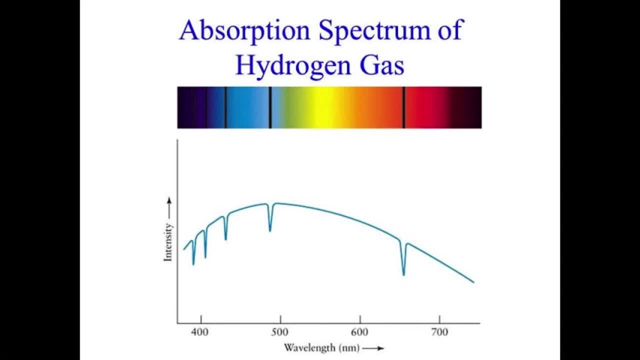 So we can record the energy emitted like this. This is called the emission spectra. The spectra that is recorded is a plot. We can take the intensity, absorbance or transmittance in the x-axis. In the y-axis, we can take the wave number or wavelength. 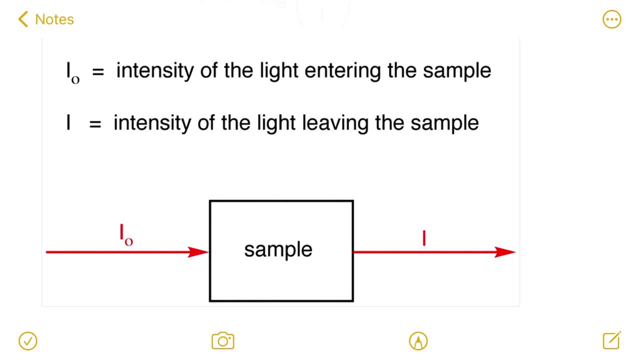 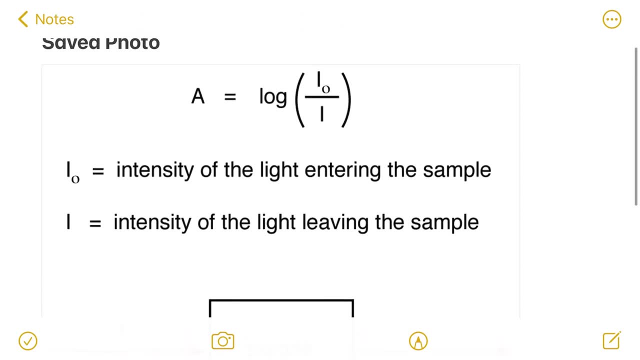 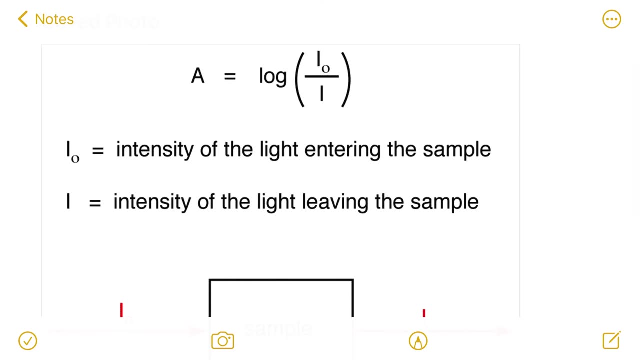 When the light with an intensity of i0 enters the sample, the light with a different intensity of i will come out of the sample, Because a certain amount of light has been absorbed by the sample. To calculate the absorbance, we have an equation that is: 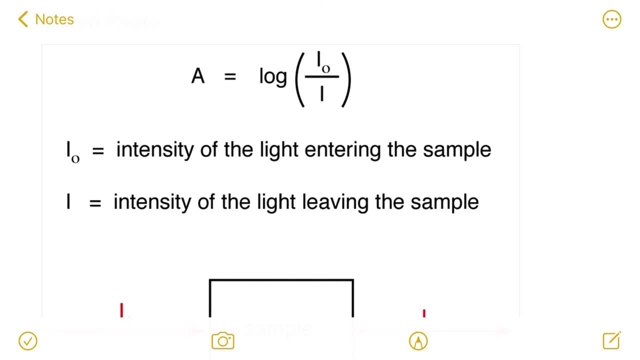 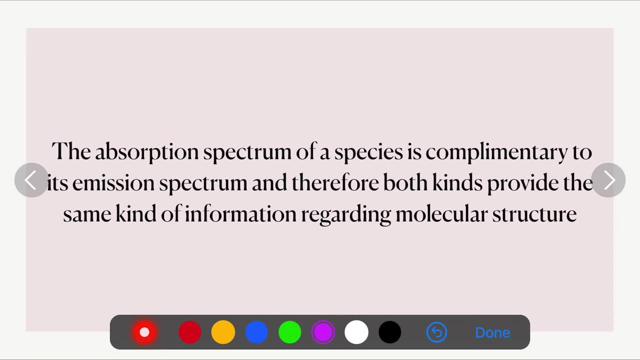 a is equal to log i0 by i. When we examine the spectra of different molecules, the shape and appearance of each spectra will be different. That means the spectra is one that gives the characteristic parameter of each molecule, So we can give a very valuable information about the structure of each molecule. 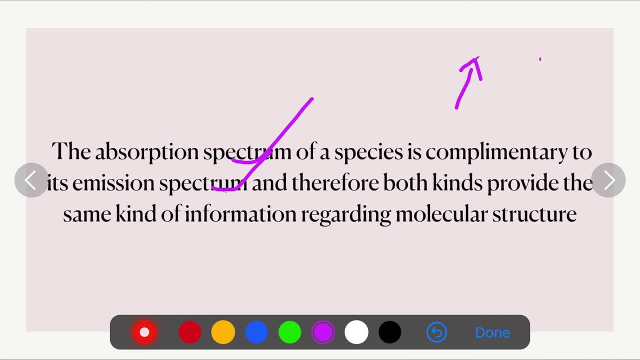 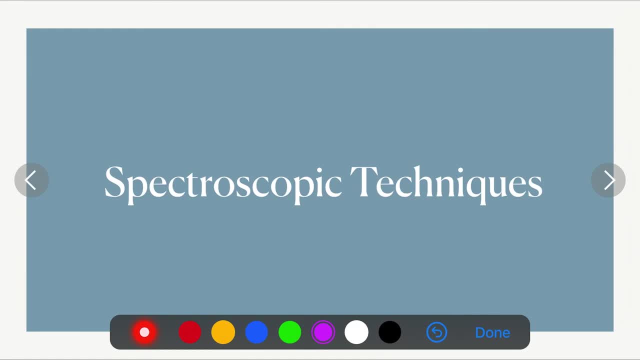 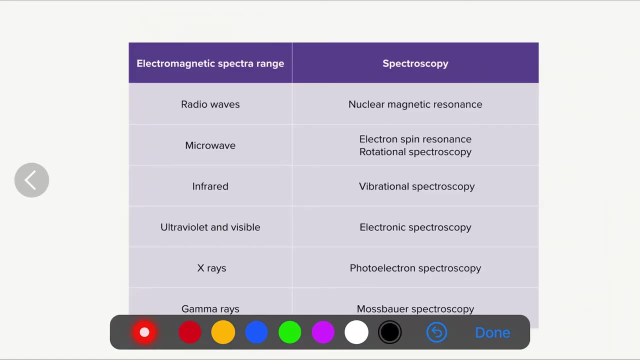 Whether it is an absorption spectra or a complementary emission spectra. So on the basis of which frequency the molecule absorbs the energy, we have different kinds of spectroscopic techniques. If our molecule absorbs electromagnetic radiation in the radio frequency region and conducts the transition, 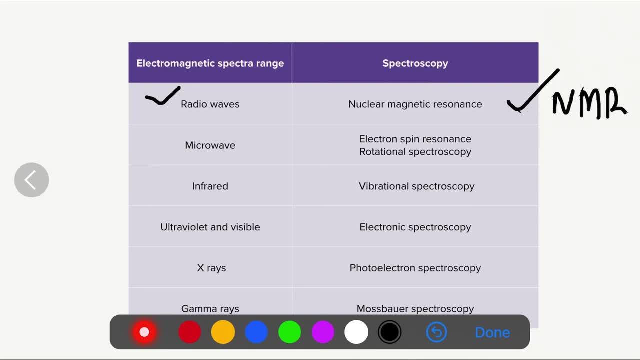 we have this nuclear magnetic resonance. The other one is the resonance spectroscopy, that is NMR. If the absorption is done in the microwave range, we have this resonance spectra, that is, electron spin resonance spectra, And another one is rotational spectra. The absorption in the infrared range is a transition in the vibrational energy levels of our molecules.